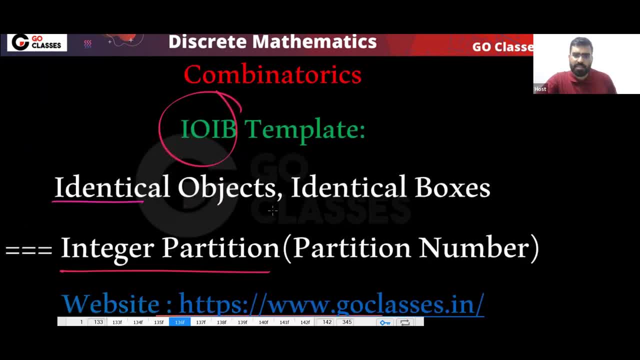 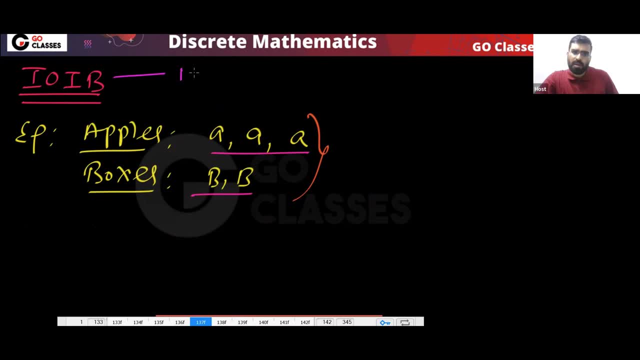 also same and boxes are also same. Identical objects and identical boxes. Both are identical. Now tell me how many Bs will be there. Again, there is no formula for this. Again, there is no formula. So what we should do, What you should do, 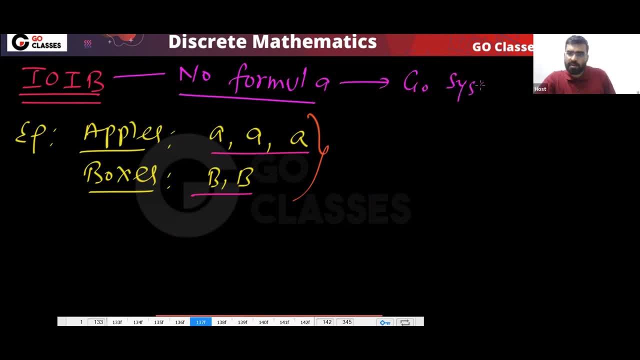 For this. So go systematic, Go systematic way. This is what you should do, Always go systematic way. So what will be the systematic way? Using one box like one part. So again, you can go in a systematic way. If you only do, one part means only one box you use. then 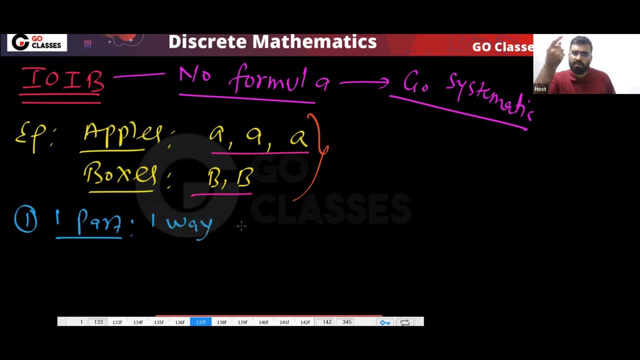 only one way, Then only one way. Okay, Only one way because all the apples will be together. Boxes are same, So it does not matter which box you choose. Boxes are same, So only one way. Next, if you use two, part means because two boxes you have, So how many? 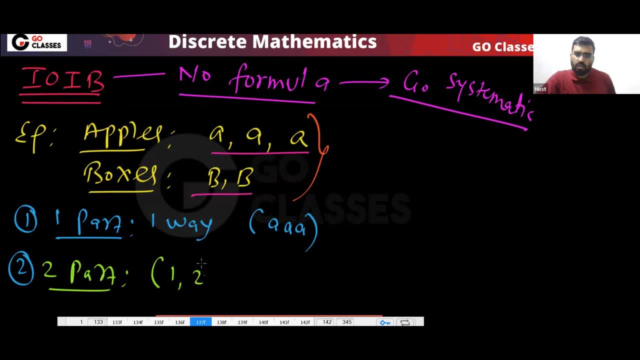 ways are there, Then? how many ways are there? One comma two? Only this, Tell me. one comma two. How many ways are there for one comma two? Only one, Only one way, Because, remember, all the apples are same, All the objects are same, All the objects are same, So only this. 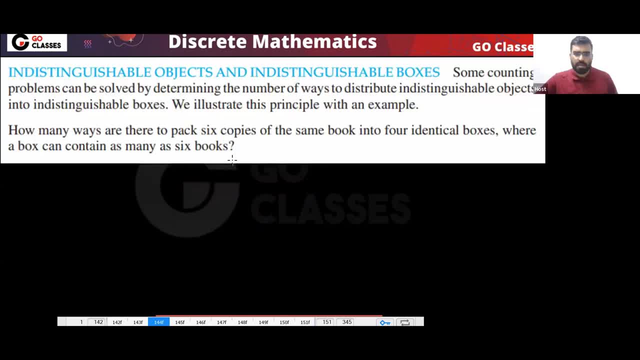 you can do Nothing else. you can do Very simple, Right, Let's see this question. So there are six copies of the same book and four identical boxes. Okay, Any box can contain any anything. So there are six copies of the same book. Now tell me what will be the answer. 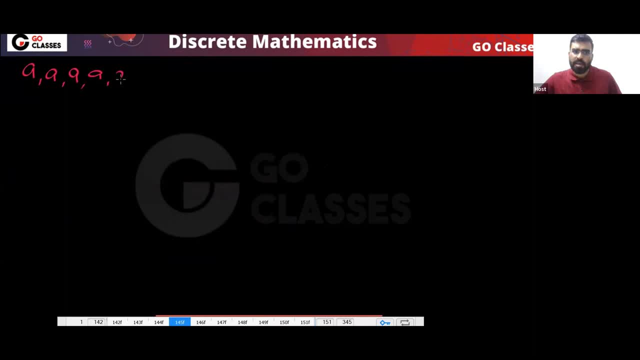 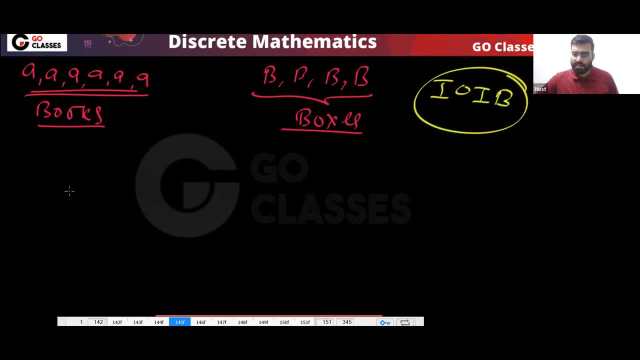 I O I B. Template. I O I B. Identical object, identical boxes, a template. So what will you do? Always go in a systematic way. So only one part, If you only use one box. if you only use one box, then how many ways? If you only use one box, then how many ways? 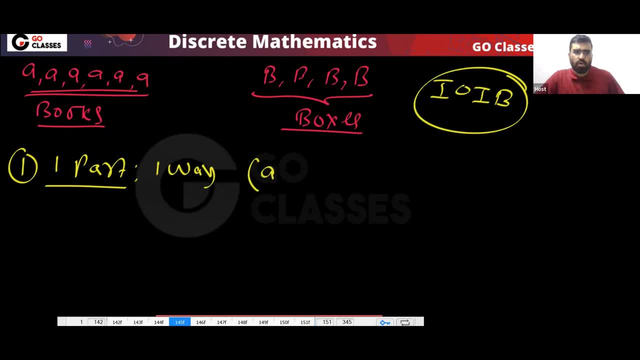 Only one way. Only one way. All will be together. All six will be together. All six will be together. All these six items will be together. Okay, All these six items will be together. Okay, If you want to create two part, then if you want to create two part, then then. 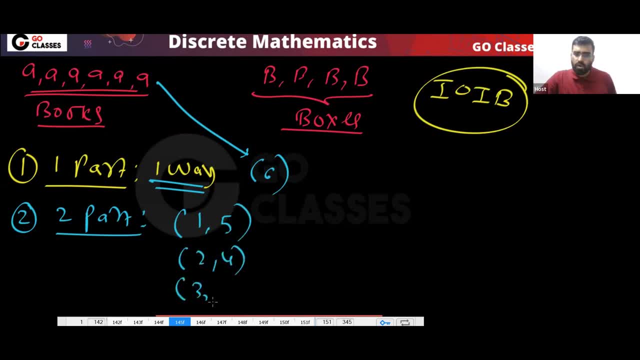 you can create 1 comma 5, or you can create 2 comma 4, or you can 3 comma 3.. Only these, you can create, Only these. How many ways here. How many ways here, Again, only one way, Again, only one way, Again, only one way. So this, I, O, I O, I. B template is very. 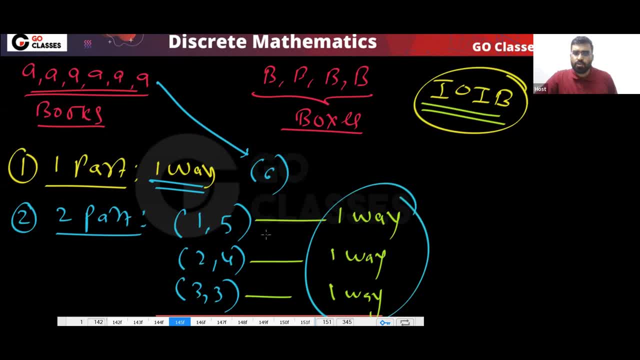 simple right. You don't even have to calculate. You don't even have to calculate Always. you will have one way, because all the objects are same, All the all our apples, all our apples. It does not matter which apple you put separate, All apples are same, All apples. 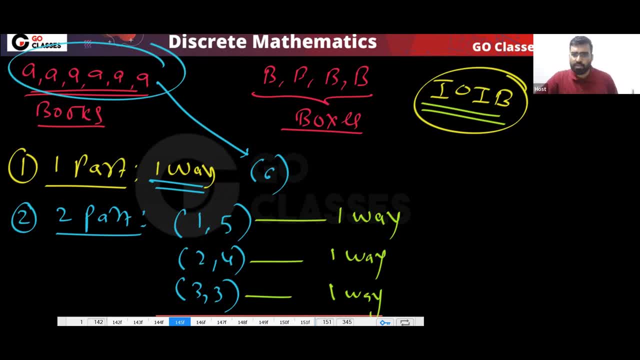 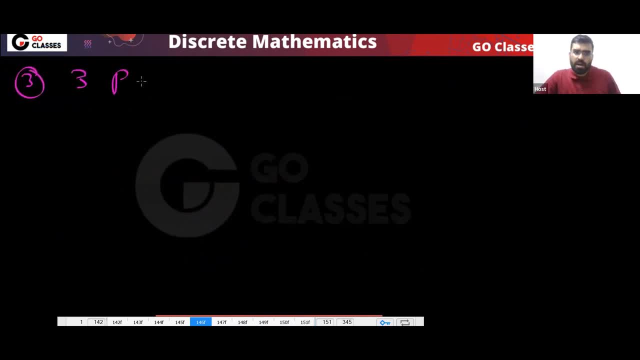 are same. It does not matter which apple you put separate. It does not matter, Just write the cases. Every case will have only one way: The third three part. How many three part partition are there? If you use three part, then you can do 1 comma, 1 comma, 4, you can. 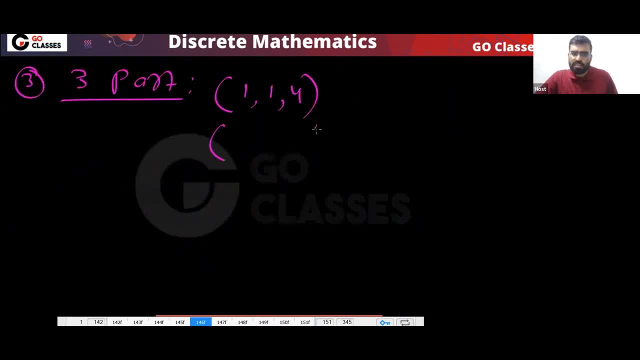 do So. you can do 1 comma 1 comma 4, go step by step, go step by step. or you can do 1 comma 2 comma 3, you can do, Or what you can do. You can do 2 comma 2 comma 2, you can do Is. 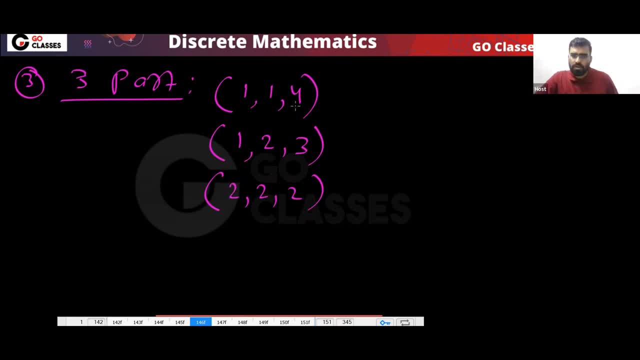 there anything else? 1 comma, 1 comma 4, or so step by step you go. So this is your 1 comma, 1 comma 4.. Now what you do? 1 you give here, So 1 comma, 2 comma 3.. Another situation: 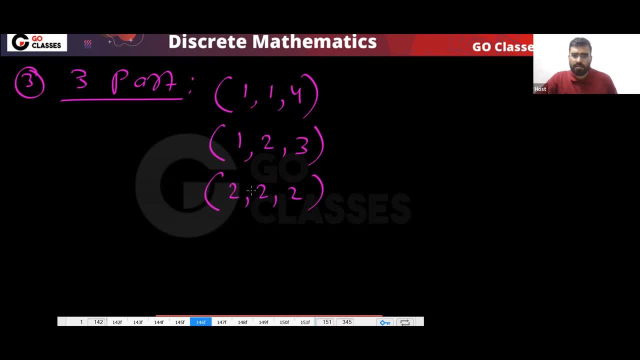 if you give this here, then nothing will happen. So this is your 1 comma 1 comma 4.. Now what you will change? 2 comma 1 comma 3. Because if you give one here, then it will change. 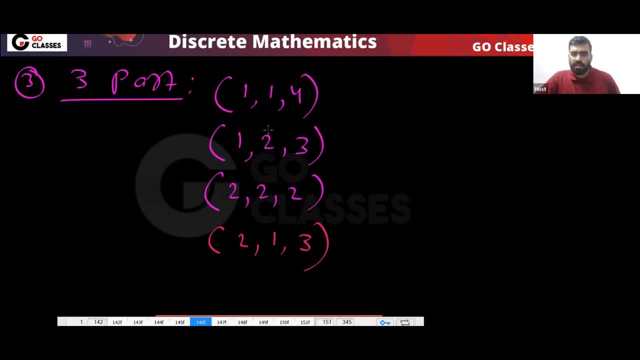 You will see, If you give one here, then you will get 1 comma 2 comma 3.. If you give this here, you will get 2 comma 1 comma 3.. No, 2 comma 1 comma 3 is same as this. So these: 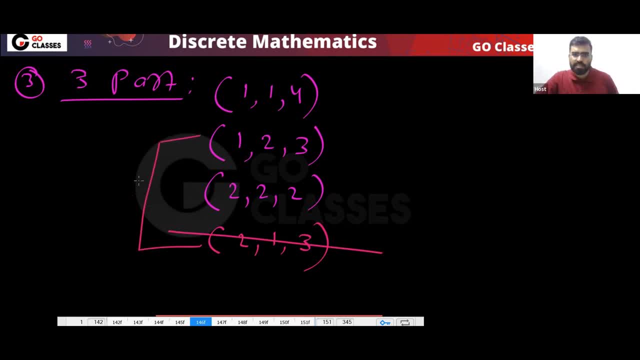 are same. This 2 comma, 1, comma 3, this is already counted. These two are basically same. So there is no difference. Only one way. Only one way, Very simple. Next And next 4 parts, Because you have total. 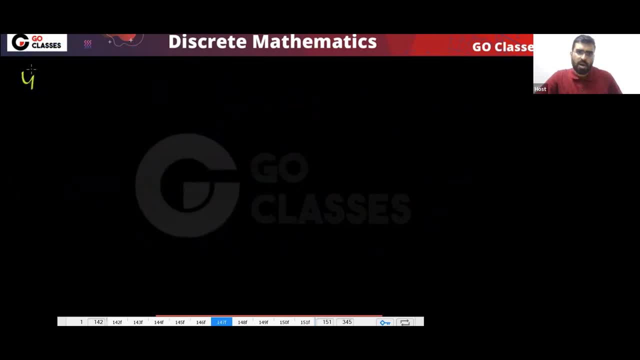 4 boxes you have, Because you have 4 boxes. so 4 part, How many, 4 part, 4 part. So means 1 comma, 1 comma, 1 comma 3, you can do, Or what you can do. You can give 1 here, So you can. 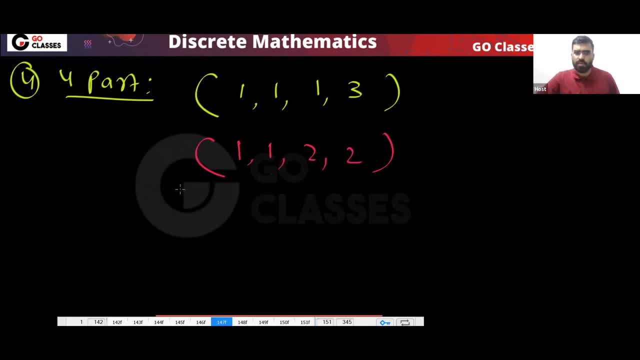 get 1 comma, 1 comma, 2 comma 2, you can get Nothing else. you will get Nothing else. Again, one way, Again, one way. So the answer is very simple. What is the final answer? What is the final answer? Can you create 5 part? Can you create 5 parts? No, Because only 4 boxes. 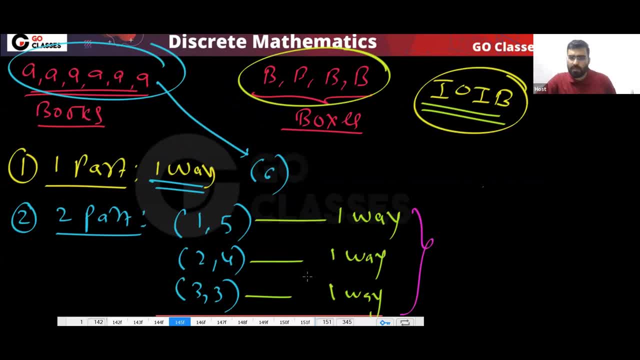 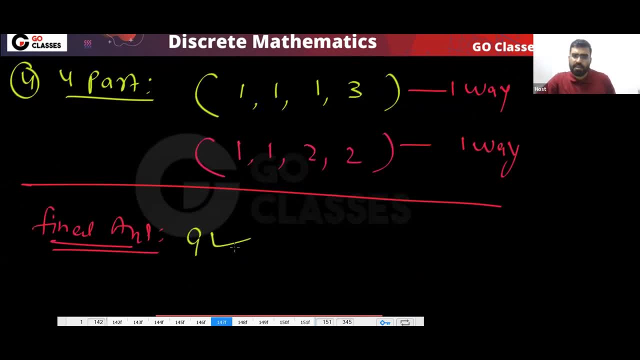 we have Only 4 boxes. we have, So you cannot create 5 parts. So the answer will be 4, 4 and 3, 7.. 7 and 2, 9. The answer will be 9.. So this is very simple. Now another question. 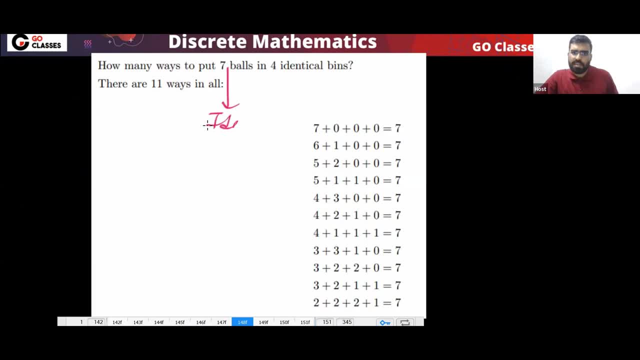 7 identical balls. So let's assume you have 7 identical balls And 7 identical balls and 4 identical bins. Then number of ways, Number of ways. See, don't follow this. Actually you should follow the systematic way: How many one part partition you can create, So one. 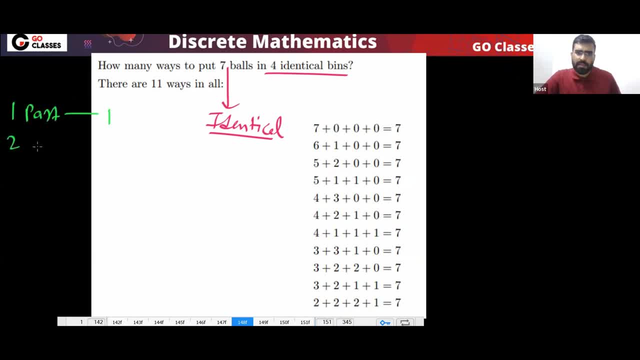 part, only one, One part, only one. Next 2 part. How many 2 part you can create? So for 2 part, Because you have total 7 balls. So 2 part will be like this: 1 comma, 1 comma, 2 comma. 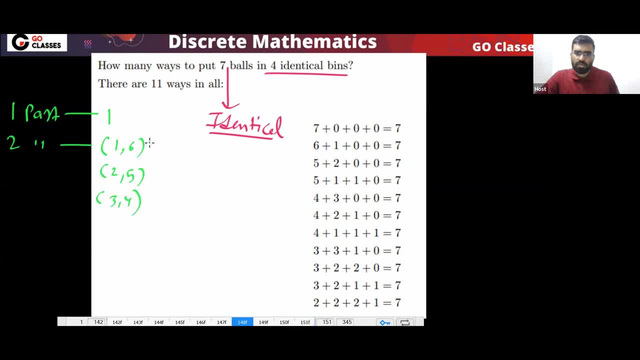 1 comma, 6.. 2 comma, 5.. 3 comma, 4. So there will be 3.. There will be 3.. Next then you can count how many 4 part, How many 3 part will be there. So 3 part will be like this: 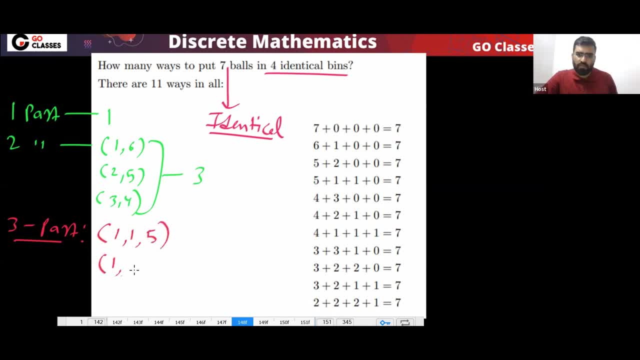 1 comma, 1 comma 5.. Or I can do 1 comma, 2 comma, 4.. Or I can do 2 comma, 2 comma 3. So 2 comma, 2 comma 3.. Anything else can I do. I think 3 comma, 3 comma, 1, that also I can do, 3 comma, 3 comma. 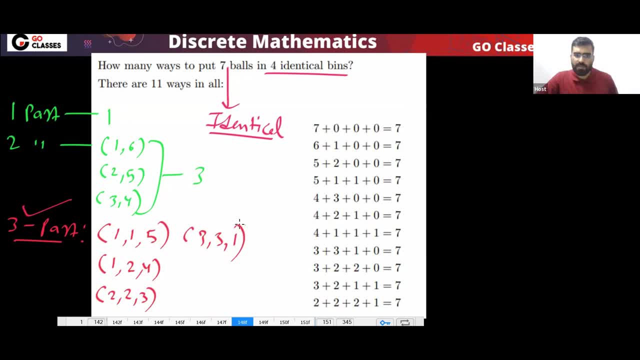 1. that is also So for 3 part, there will be 4.. There will be 4 for 3 parts And finally for 4 parts. how many will be there? For 4 parts, that will be 1 comma, 1 comma, 1 comma. 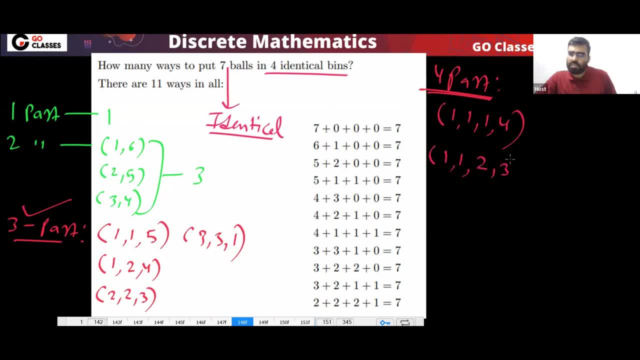 4, and then there will be 2, 3, and then there will be 1, 2, 2, 2.. Okay, You can just check it out, Right? So there will be basically 4, 3, 3, 4, 3, and then 2, 2, 2. And that's it, And there will be 2, 3, 2.. Also, you can do 6, 2, 3, 2.. Whatever. 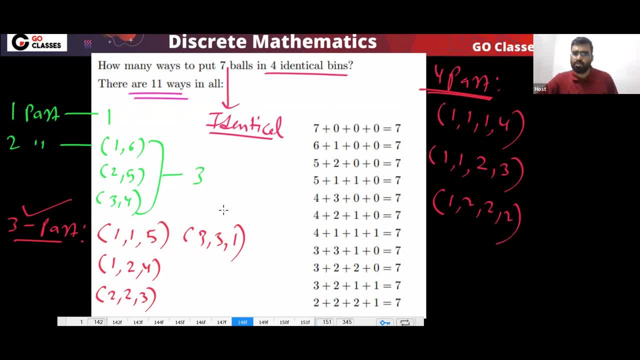 I think that will do. Ok, then Go ahead and check it out. Alright, Then now I am عن and 1. So the answer will be 11.. So like this you can do Very simple, right? Okay, So these. 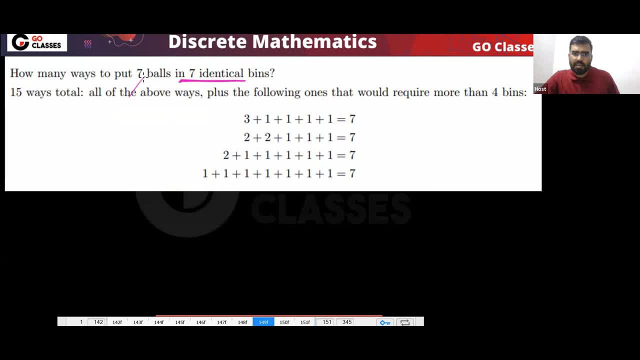 questions are very simple. And if you have 7 identical bins- if you have 7 identical bins- then some additional things will be there, So you can just calculate. If you have 7 identical bins, okay, then you will have to find how many 5 part, how many 6 part, how many 7 part. 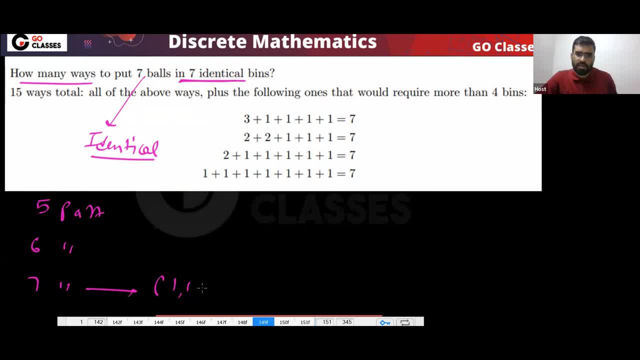 7 part will only be 1.. 7 part will be like this: 1, 1, 1,, 1, 1, 1.. So that will be only 1.. Only this you will get. 6 part also will be there: only 1.. Like this, you will get This. 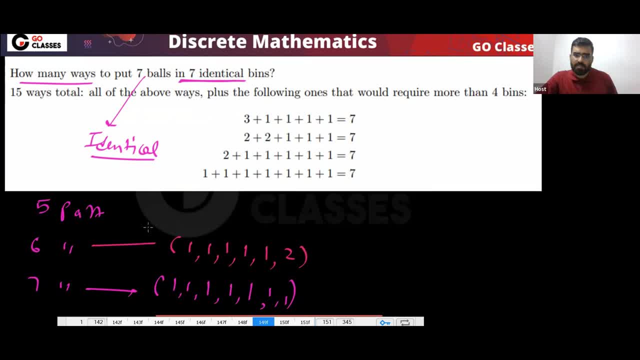 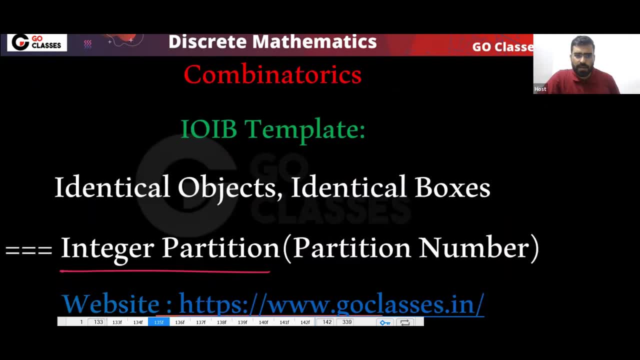 is your 6 part? Okay, this will be your 6 part, And how many 5 parts you will that you can count? Okay, how many will be there? Is this clear Now? the next concept is integer partition. We have already seen integer composition. 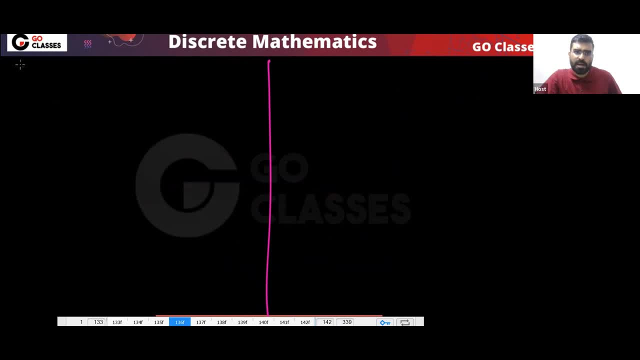 So what is the difference between integer composition and integer partition? So you know that integer composition of 4.. Let's find out. Let's find out composition of 4.. What is composition of 4 and what is partition of 4?? What is partition of 4?? So integer composition. 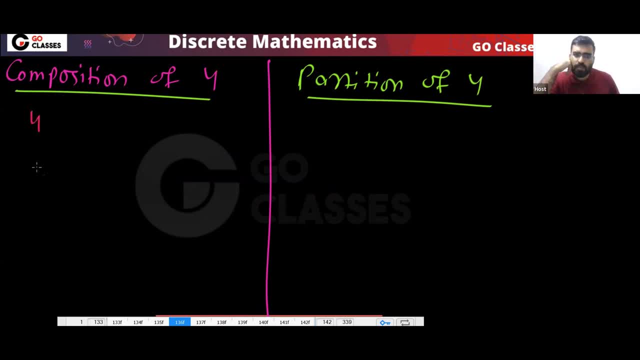 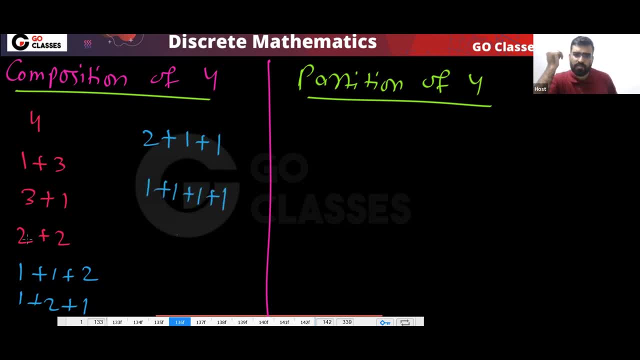 also composition. And then finally one plus one plus one plus one: this is also composition, But in the partition, in the partition, remember, in the partition order does not matter, In, In the partition order does not matter, In the partition order does not matter. 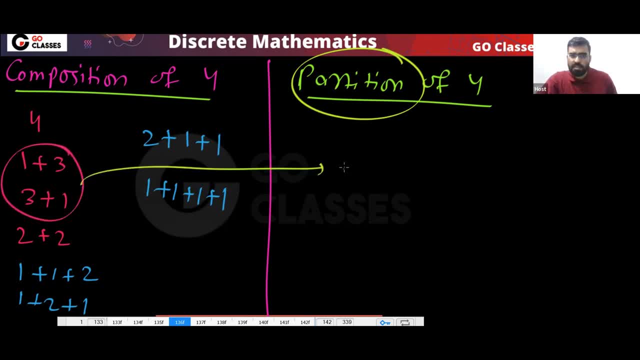 So in the partition, these two things will become same here. These two things will be same here. Just only one. These two things will be only one. So this is a partition. This is a partition. This is a partition: two plus one plus one. 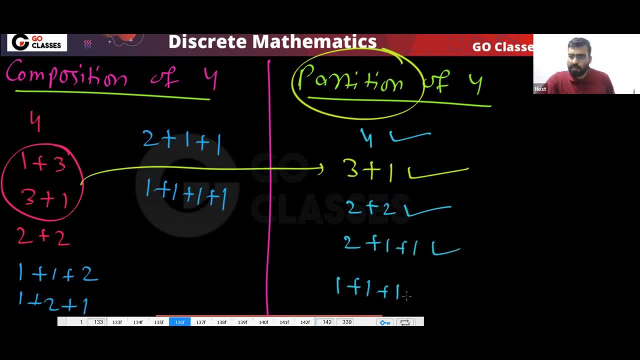 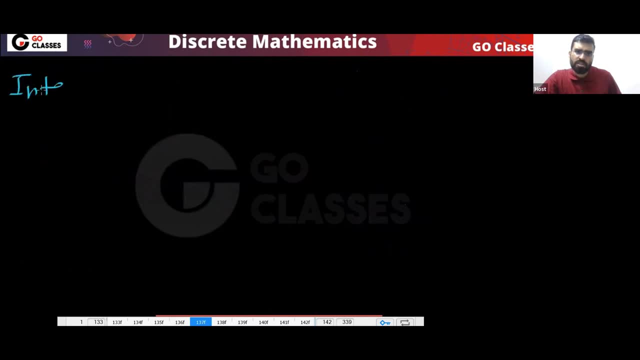 This is a partition. and one plus one plus one plus one, This is a partition. So this is the only difference. There is no other difference. So what is the difference between integer composition and integer partition? This integer composition of n. This integer composition of n. 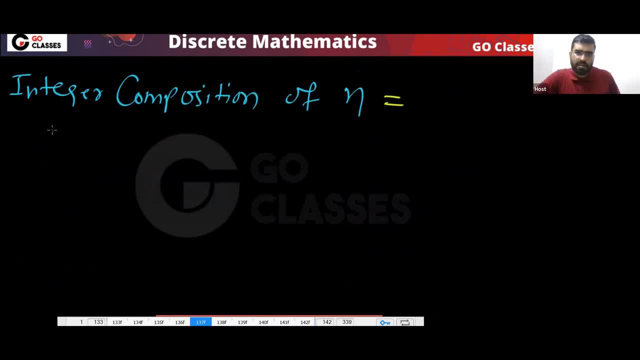 What is that? That is basically an ordered summation. This is your ordered summation. This is the difference. This is ordered summation of positive integers. So this is ordered summation of positive integers And what is integer and what is integer partition. 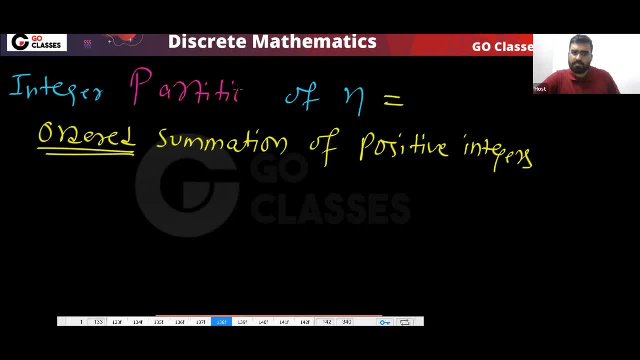 What is integer partition? This is simply unordered. Order does not matter. This is simply unordered, So order does not matter here. Order does not matter here. So this is the partition and this is the composition, And this integer composition, this problem, it follows what template. 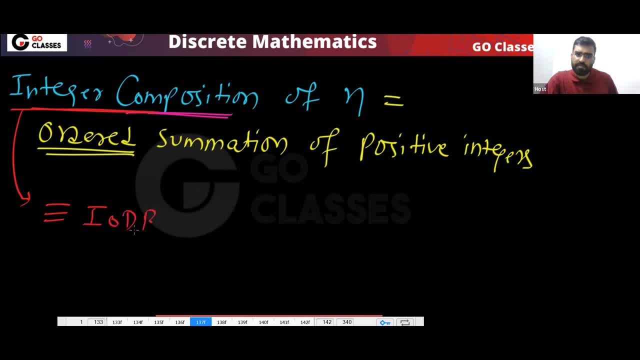 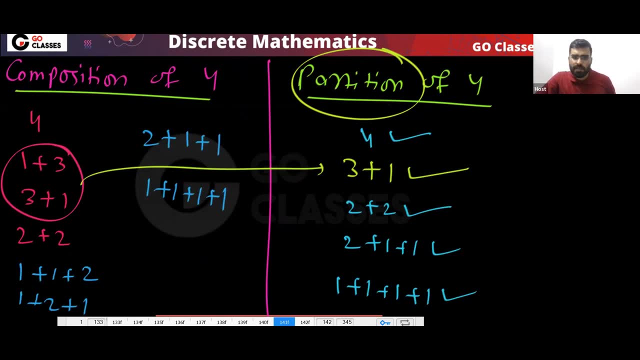 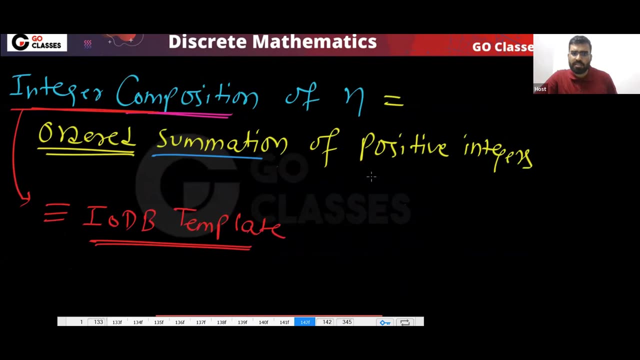 This problem follows. what template? Iodb template. This will follow Iodb template. Now I told you that what is composition and partition? This difference? I was telling you the difference between composition and partition. So composition is basically ordered summation. This is the orded summation. 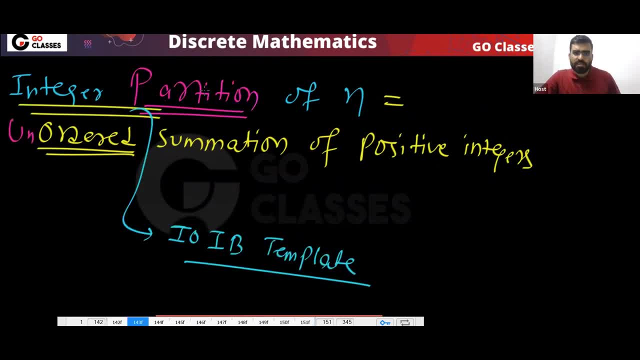 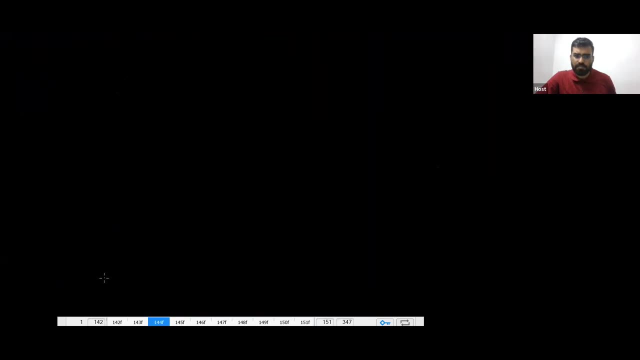 This will follow Iodb template, But you can notice this: integer partition of n. integer partition of n, that is, unordered summation of positive integers. This will follow Iodb template. What it means? it means like this: This will follow Iodb template. 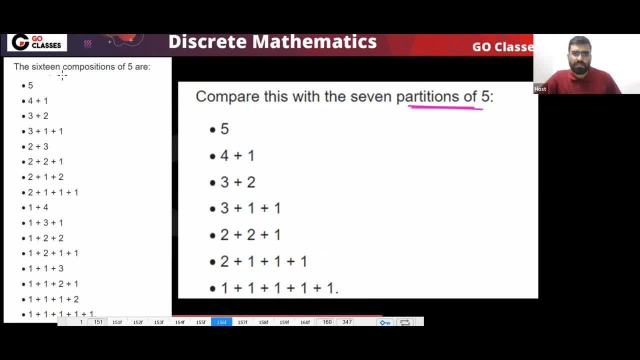 So first you understand the difference between partition of five: These are the partition of five and these are the composition of five In a partition. order does not matter Order- this is unordered, This is unordered submission, So order will not matter. So, because order will not matter, 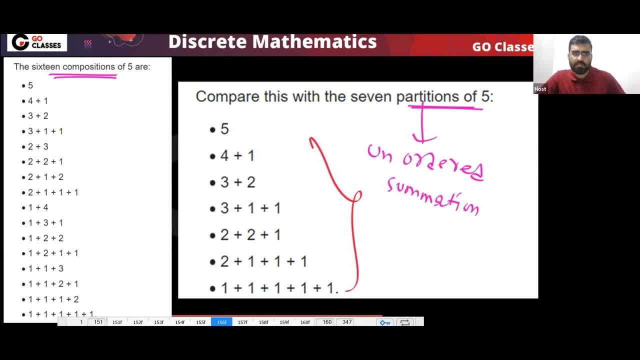 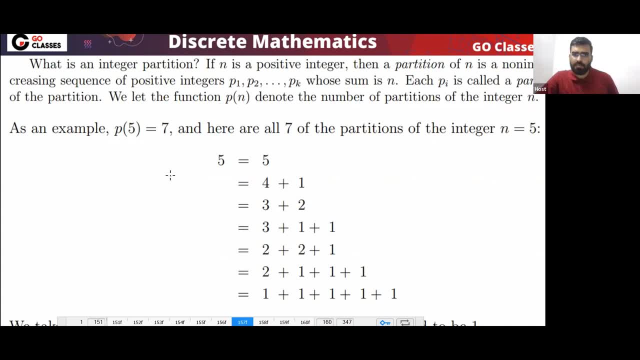 So you will have. these are the partitions, only these partitions you can create. Okay, So, for example, what will be p5,? p5 means how many partitions of five. p5 means how many partitions of five. So, for five, these many partitions, how many partitions of number five, how many partitions? 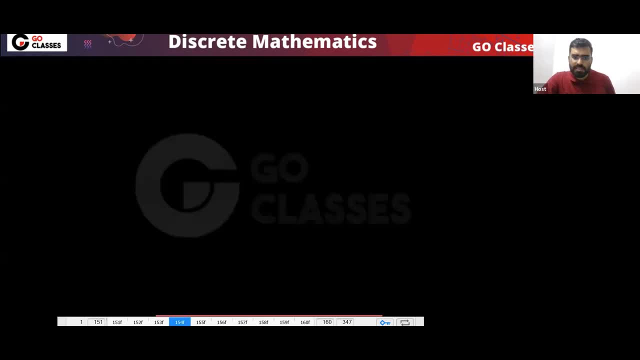 of number five are there, Remember, please? please see the difference between partition of a set and partition of a number. Please note the difference. Partition of a set. partition of a set of three elements. how many will be there? Partition of a set of three elements. 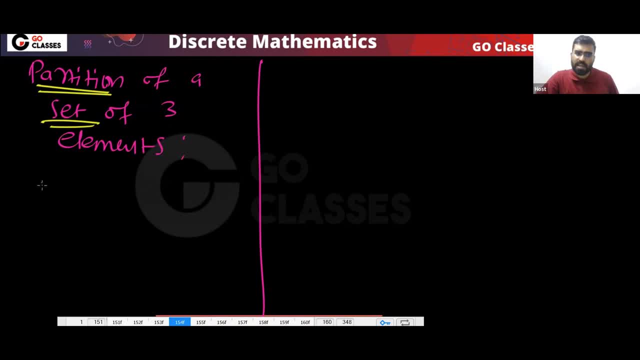 If you have a set, Okay, How many partitions will be there? If you have a set of three elements, that will be like this, like this, like this, okay, So there will be total, So there will be one way. 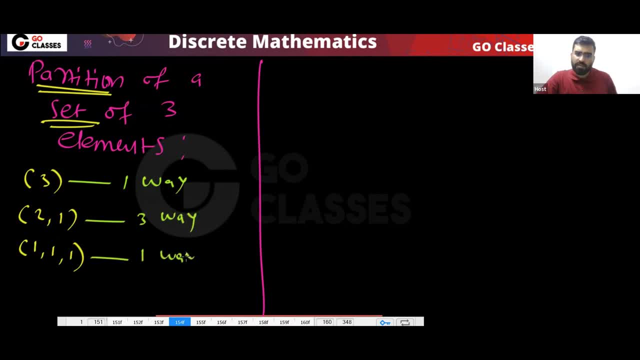 Here you will have total three way and here you will have total one way, So there will be total five. There are total five partitions, but now see, if you partition integer, partition of three means p3.. What is that? So this p3 is like this: 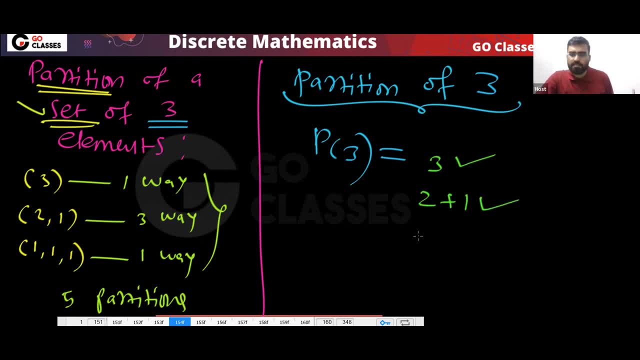 This: this is a partition. This two plus one is a partition. One plus one plus one: This is a partition. So this p3 will be three only. This is three only. So please note the difference. Is the difference clear: Partition of a set, partition of integer, partition of a set and partition of three. 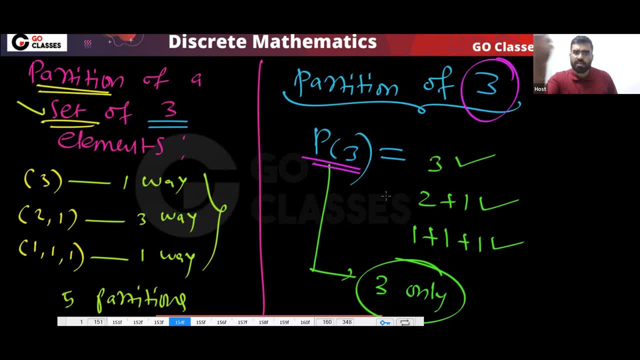 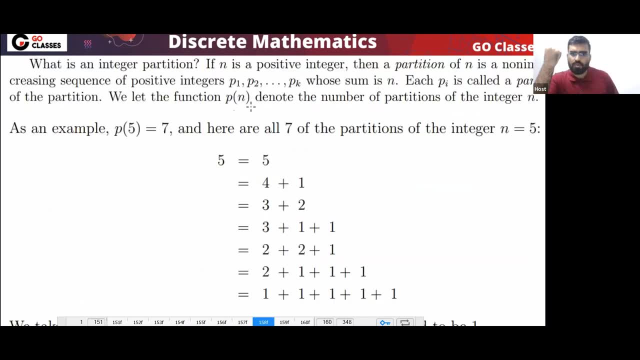 This is the partition of three. Partition of n means unordered summation, So okay, So basically, these, like these, are the partitions of five. Okay, So is this idea clear? p5, p5 means how many partitions of five are there? 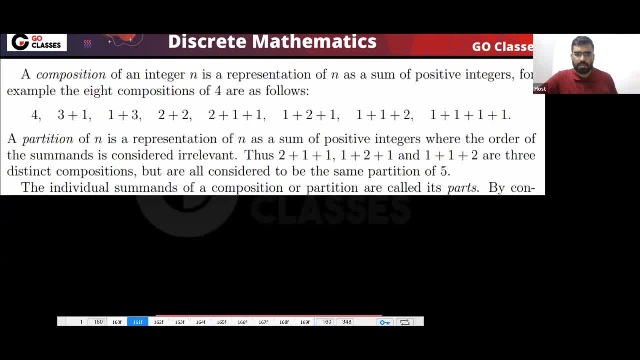 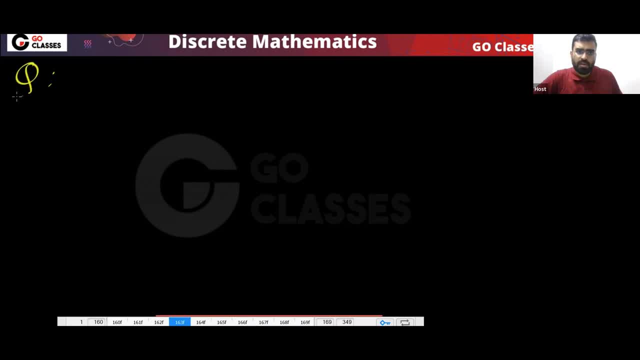 Okay, Now one thing: you note that if I ask you how many partitions of six are there, then how will you find? If I ask you how many part, If I ask you p6. What is that? That is basically integer partition of six. 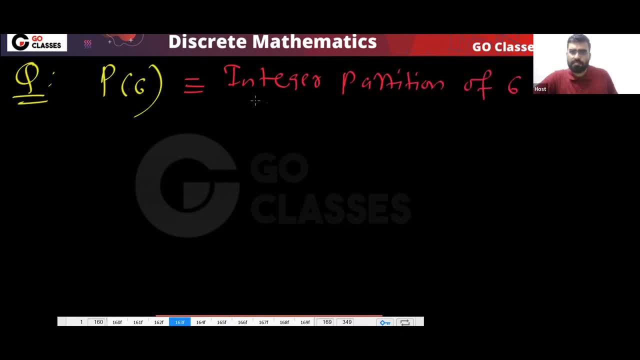 That is integer partition of six. Then how will you find? Just think about it, How many? Okay, Because you want. this is unordered. Order does not matter. Order does not matter, So this is unordered. This is your unordered summation. 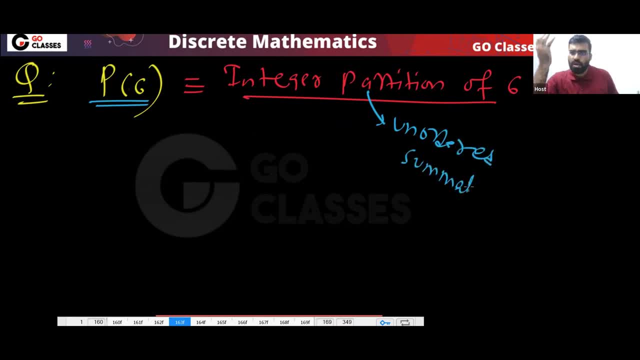 Unordered summation. So if I ask you, how will you find this? This is unordered. How many partitions of six are there? Then just go step by step, just go step by step, like only one part, Only one part. This is the only. 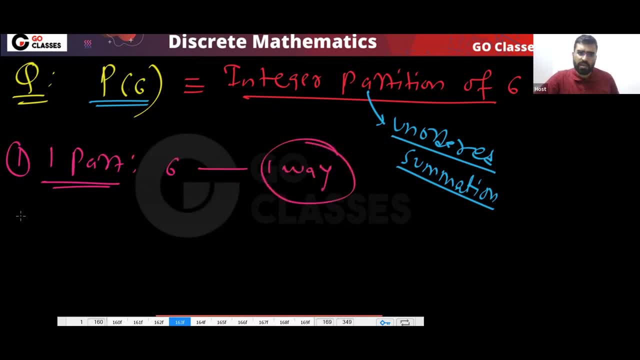 Okay, So only one way, Only one way. Okay, Because only this you can create, Only six, you can create Very simple. Then you can create two parts. If you create two parts, then one plus five you can do. You can do one plus five. 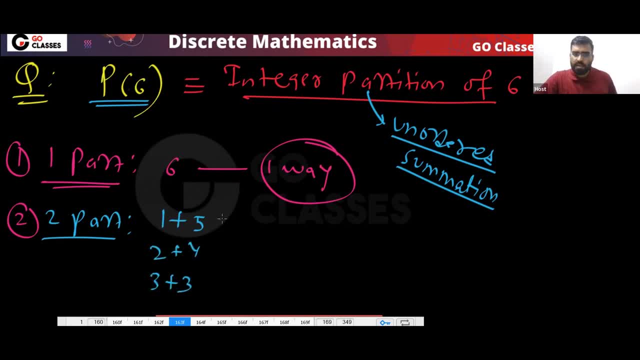 You can do two plus four, You can do three plus three. So here only one way right, Because you cannot do five plus one, You cannot do five plus one, Okay, You cannot do five plus one. So you can do one plus five, two plus four, three plus three. 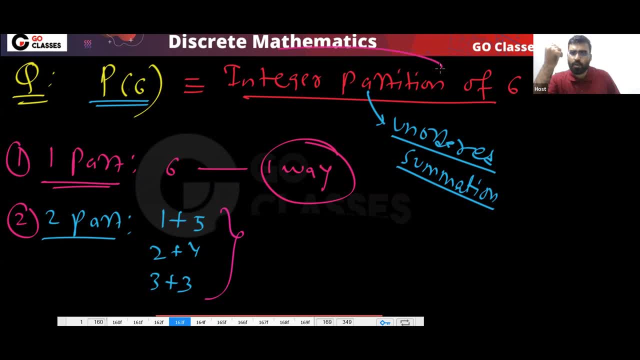 This is what you can do. So, can you notice? this integer partition problem is same as IOIB. Can you notice this? that integer partition problem is same as IOIB, Because order does not matter. So this integer partition problem, this is same as IOIB. 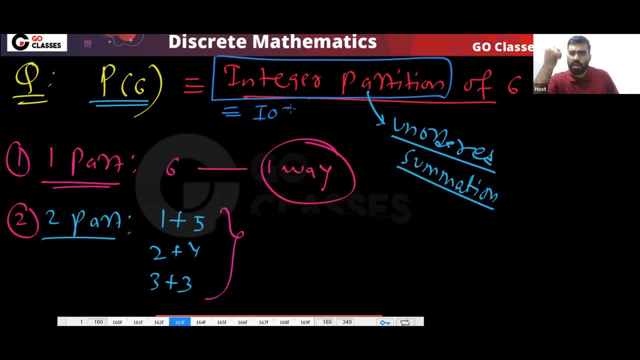 Yes or no. This is same as IOIB. Similarly, you can find three part. Okay, So how many three part will be there? So you can create like this: One plus one plus four, you can do. Or you can do one plus two plus three, you can do. 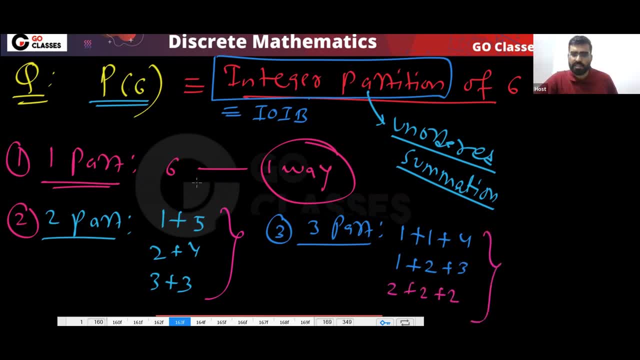 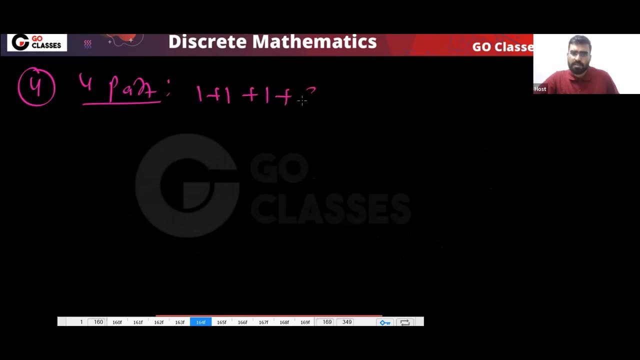 Or you can do two plus two plus two. you can do So like this. you can do: These are the three part. Okay, And then finally four, This fourth, Four, Four part. Then you can find four part, And the four part will be one plus one plus one plus three. 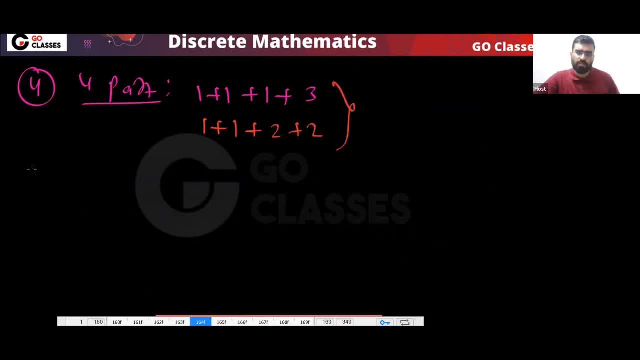 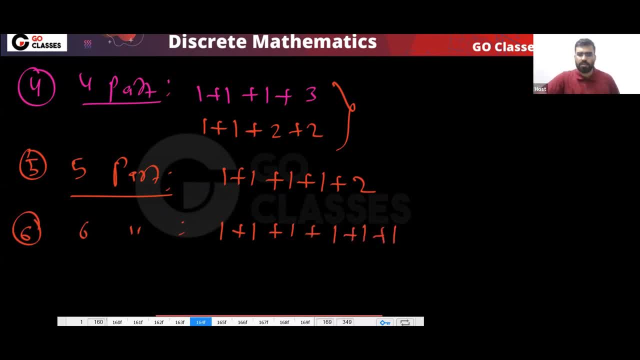 One plus one plus one. So very simple, Okay question. And this is the complete. so this is your complete distribution. So remember: partition of a set. this will follow which template. If I ask you partition of a set of a set. if I ask you partition of a set, this will follow which template. This will. 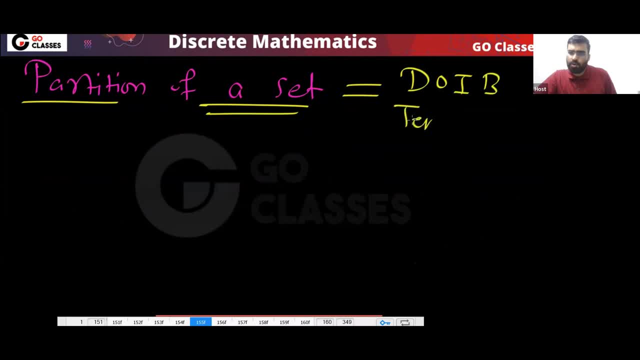 follow DOIB template. This will follow DOIB template, Okay. And partition of number and partition of a natural number: partition of a natural number: that will follow IOIB template. This will follow IOIB template, Okay. so partition of a set: we have already seen this. 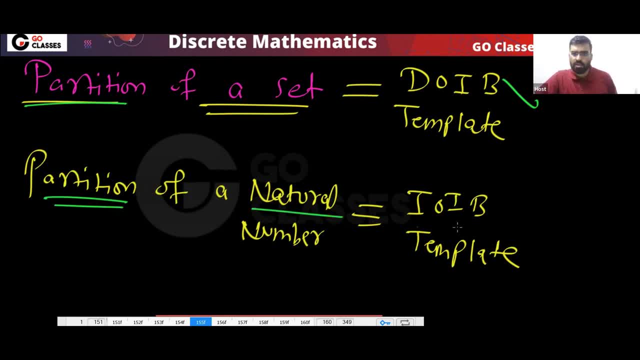 DOIB: partition of a and this natural number. that will follow IOIB template and composition follow which. which template will be followed by composition of a natural number. and partition of a set, Which template will be followed by composition of a natural number. That is IODB. That is your IODB template. Okay, So all the variations, all the problems we have, 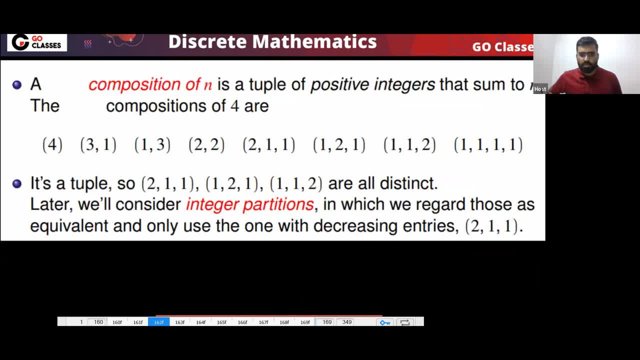 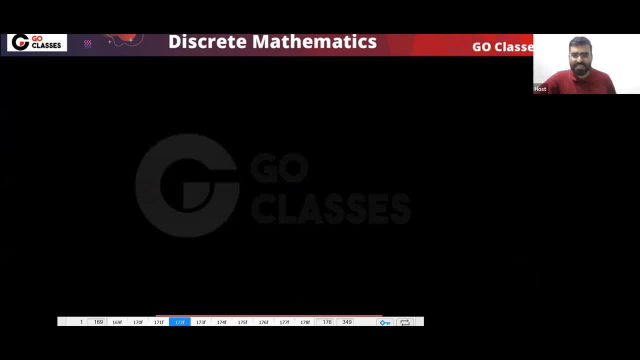 seen. Okay, this is your chapter is over. now. this basically like: okay, this was a long chapter, right? A lot of variations and a lot of things, right, Yes or no? Like: okay, this was a long chapter, right? A lot of variations and a lot of things, right? Yes or no Like?